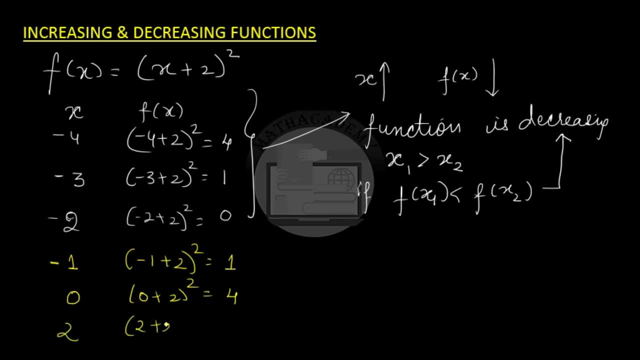 When x increases to 2, we will get 2 plus 2 whole square, which is basically 16.. So what do we see? that here, after minus 2, as x is increasing from minus 1 to 2, we see that our fx is also. 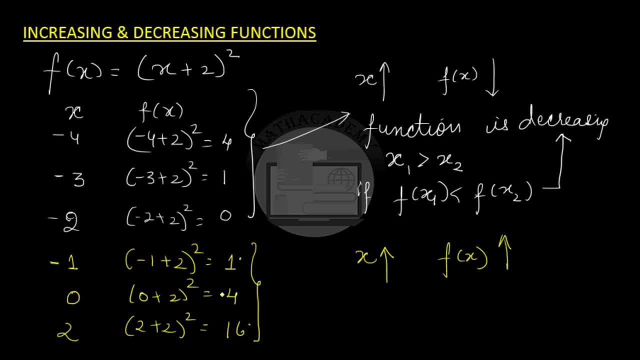 increasing from 1 to 16.. Correct, So we see that when x1 is greater than x2, then f of x1 is also greater than f of x2 and therefore in this part the function is an increasing function And the turning point where the function is changing from increasing to decreasing- 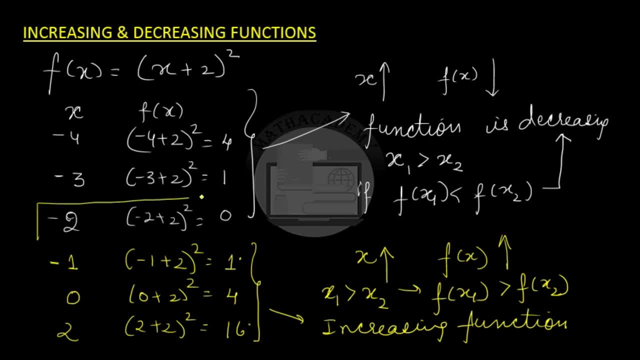 is at x is equal to minus 2.. This is the point where the fx is becoming 0 and after this it is increasing, and before this it was a decreasing function. So this minus 2- x is equal to minus 2 is called the turning point. So this is the turning point. So this is the turning point. 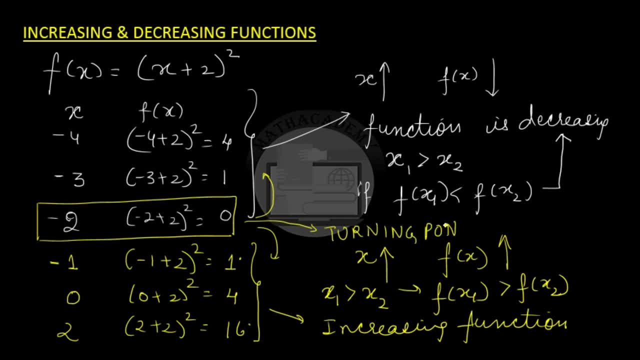 Okay, Now a turning point can be relative maxima or it can be a minima. In this particular example, x is equal to minus 2 becomes the point of minima, That's the point where the value of fx is minimum, which is 0.. Now let us understand this through a graph. 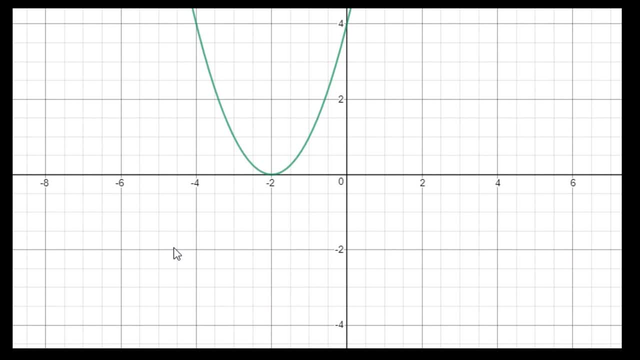 So this is the graph of y is equal to x plus 2, whole square. As I have mentioned before, we see that value of x increases from minus 4 to 2.. So the value of fx is decreasing from 4 to 0.. 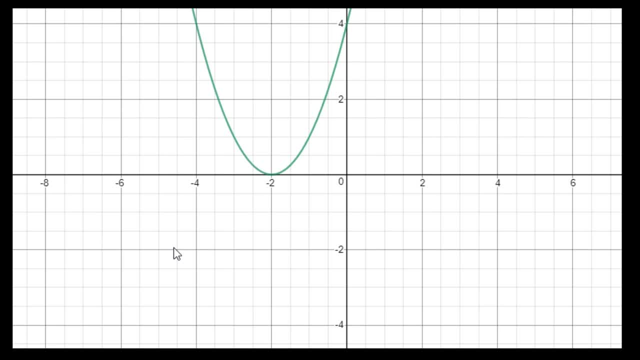 And as we go ahead of minus 2, as the value of x is increasing, we see that the value of fx is also increasing. So from minus 4 to minus 2, we see that our curve is basically a decreasing function And after minus 2 it becomes an increasing function. So at minus 2 our curve is turning. 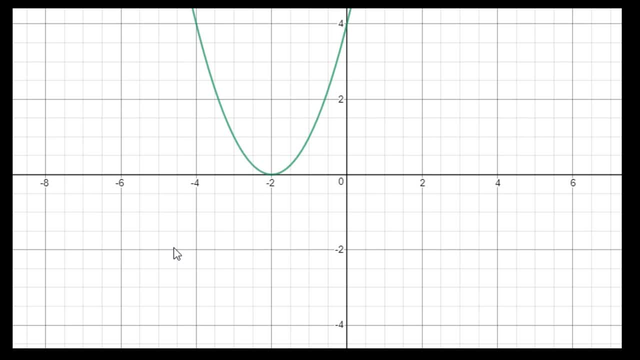 So minus 2 is the turning point and it is the point of minima, because the value of fx is minimum here. So I hope this much is clear to everyone: When is a function called an increasing function and when is a function or decreasing function? Let us see one more example. Suppose I try to 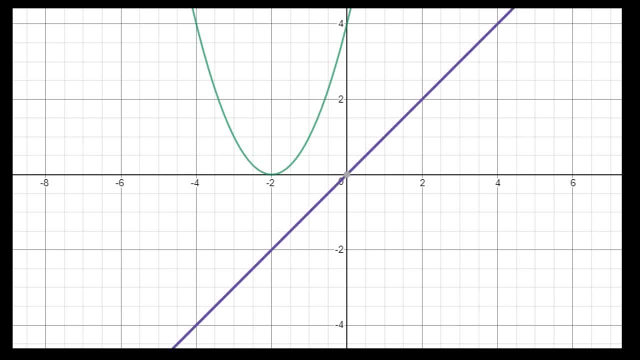 plot: y is equal to a cubic function. say x cube. The blue curve here is a curve of a cubic function. y is equal to x cube. And we see that as and when the value of x is increasing. when we move on right on the number line, the value of x increases. 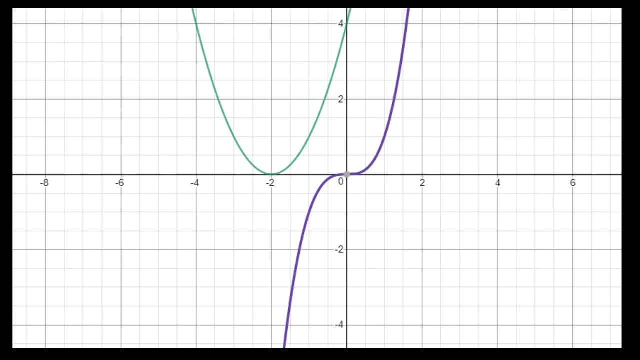 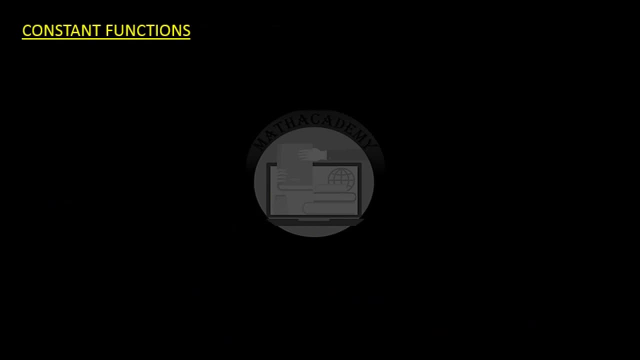 we see that the corresponding value of f of x is also increasing throughout. So we say that y is equal to x. cube, a cubic function is always an increasing function. Now let us see what a constant function is. If I write a function, y is equal to 3.. 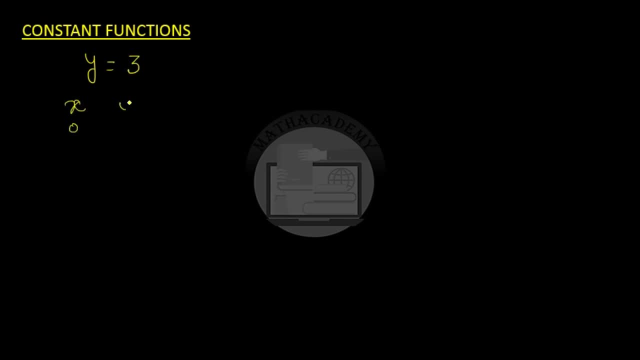 It means that whatever value of x I take, irrespective of the value of x, y always remains 3.. And when we try to plot this curve, we get a straight line which is parallel to the x axis And that straight line passes through. y is equal to 3.. 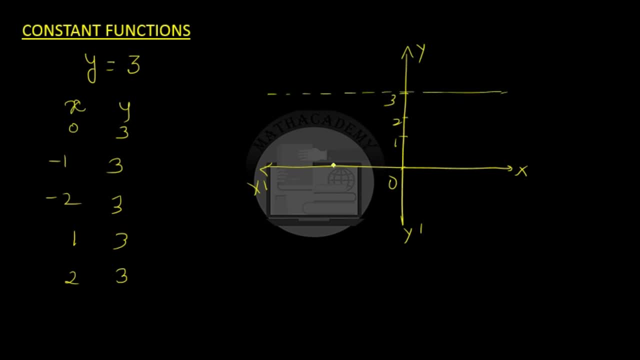 If you take a value of x here, say its x1, and a value of x here, say x2, at both of these points the value of y is always 3.. Correct At this point. at x1, the value of f is 3.. 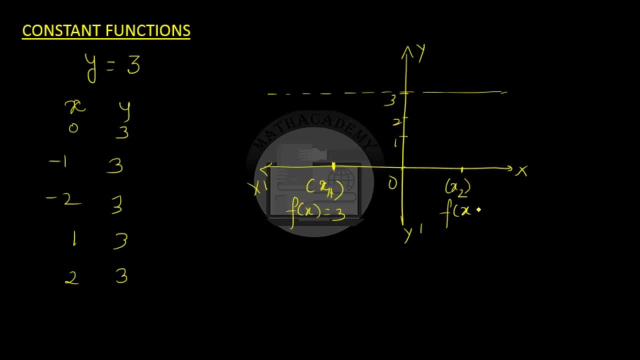 Correct At this point. at x1 the value of f is 3. And at x2 the value of f is again 3. So x1 is less than x2, but f is equal to f. If that is the case, then such functions are called the constant function. 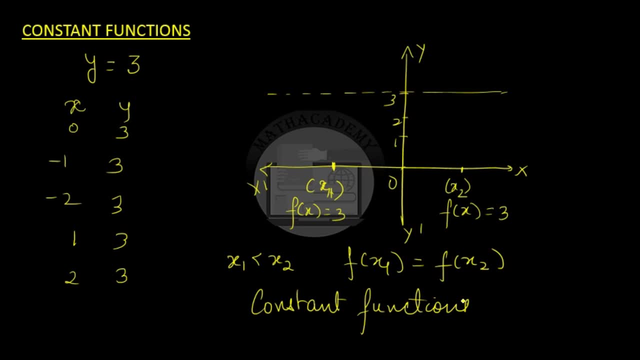 Okay, so I hope the increasing, decreasing and the constant functions are clear to everyone. In our next video we will see what are even functions, Even functions and what are odd functions. If you have any doubt regarding this video, you can send me an email at keertimathacademy at gmailcom. 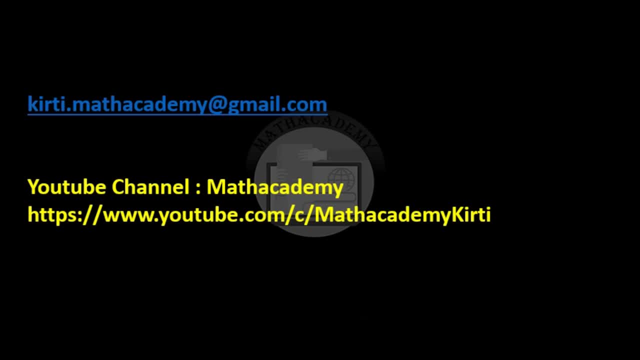 This is my youtube channel, Math Academy. If you have liked my videos, please don't forget to like, share and subscribe. Thank you.